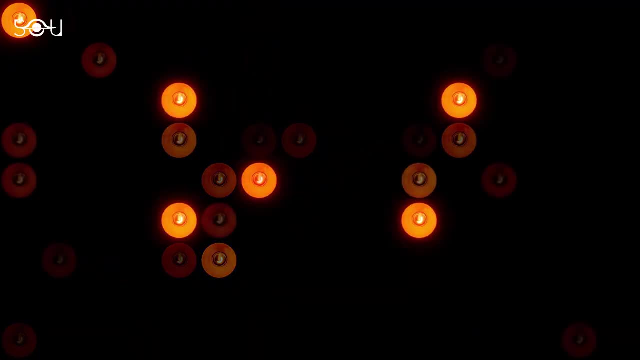 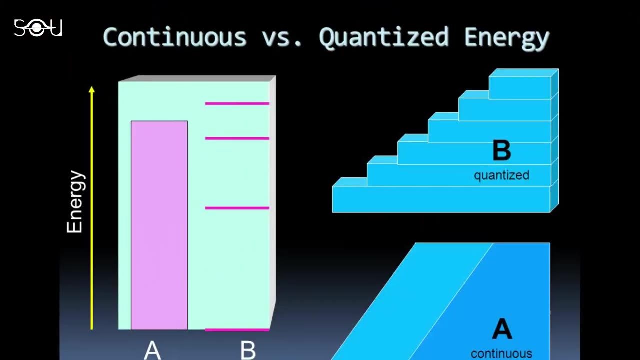 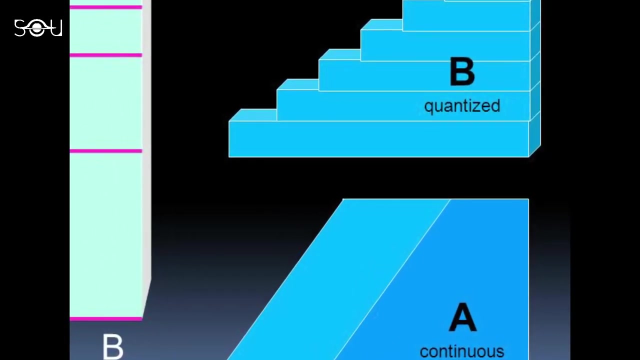 on how to solve this problem. After a lot of brainstorming he came up with an assumption. He said: energy in the form of light can only be emitted in discrete amounts. It cannot be emitted continuously. So 1.4 units, 3.5 units, 6.2 units, etc. were not allowed Planck. 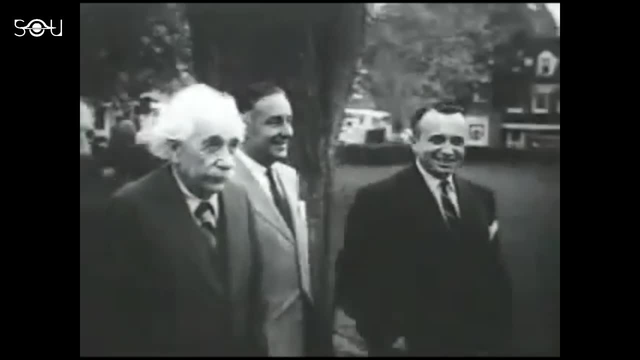 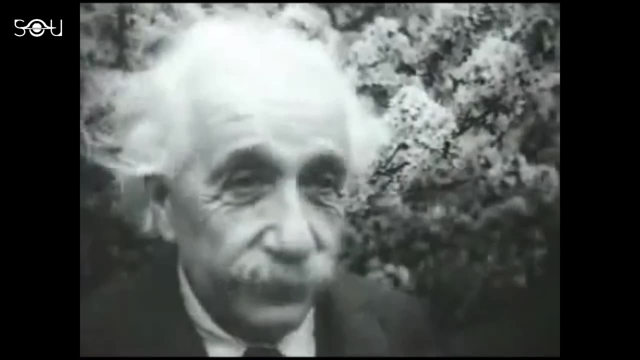 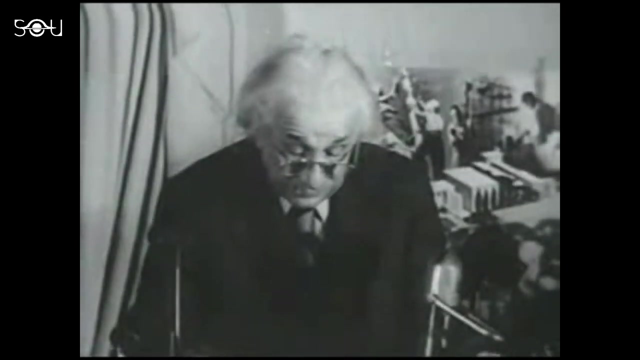 did not realize the importance of this hypothesis. Five years later, Albert Einstein, who back then was a struggling third class patent clerk in Switzerland, realized the importance of Planck's work and used it to explain the photoelectric effect. This was the second. 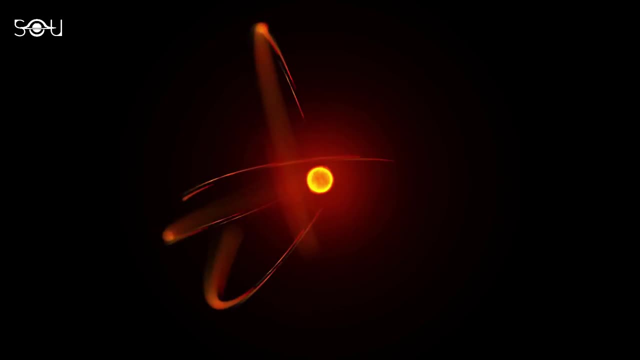 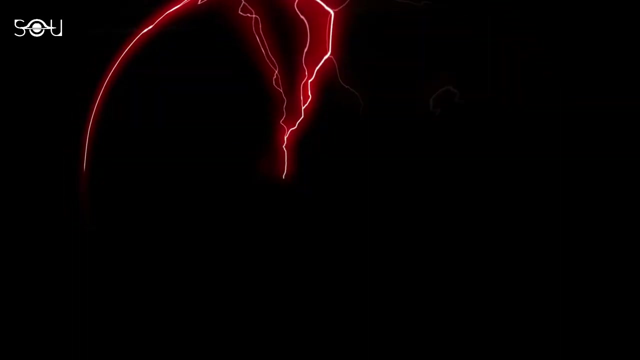 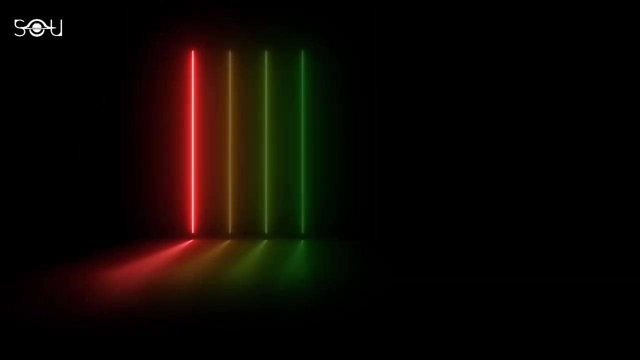 blow to classical mechanics. The third and the final nail in the coffin of classical physics came from Niels Bohr. When we pass electric current through gas to ionize it and observe it through a spectrometer, we see very fine spectral lines. Their origin could not be explained by the existing theories. 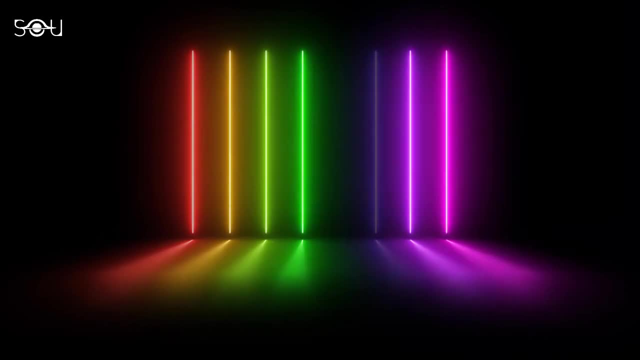 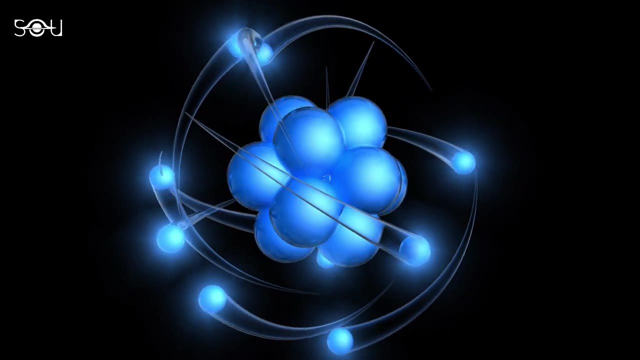 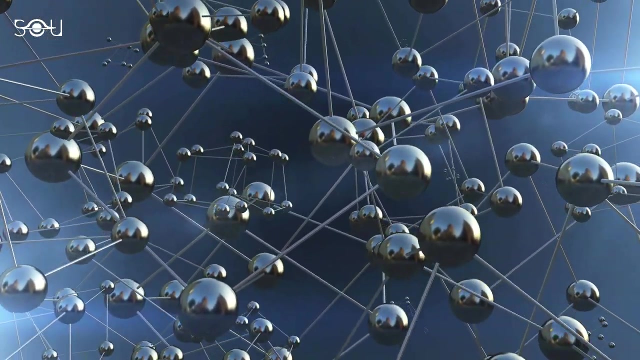 Bohr attributed these lines to the jumps made by electrons from one level to another. His theory was the first leap to explain the structure of the atom. So far, so good. But if this is what all quantum physics is, then why is it considered so weird and difficult to understand? 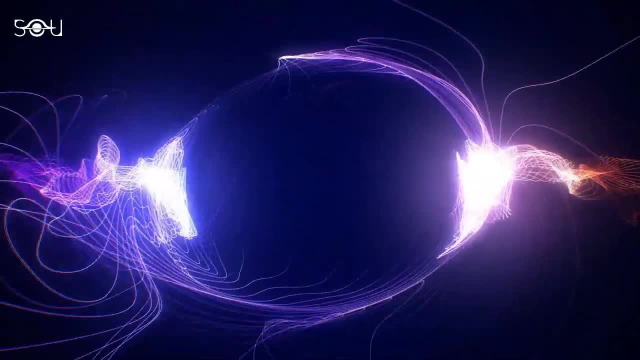 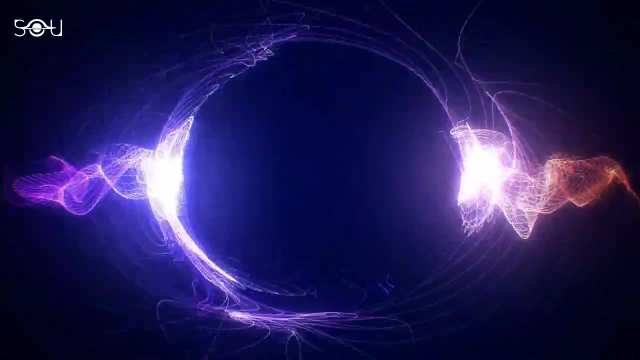 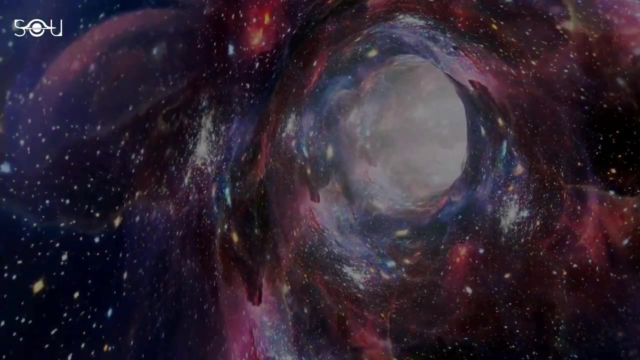 Well, the answer to this lies in the physical interpretation of some of the offbeat concepts and principles involved in this. So now let's have a look at some of the most interesting ones. 1. Quantum Tunneling. Suppose you have a bouncy ball with you and 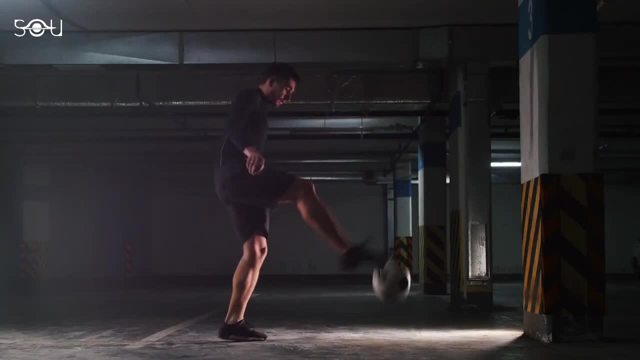 you are hitting it at a wall. What happens? It keeps on coming back to you and you keep on hitting it, But there comes a point when it just disappears at the wall and then appears on the other side of it. Spooky right. This is what quantum tunneling is. 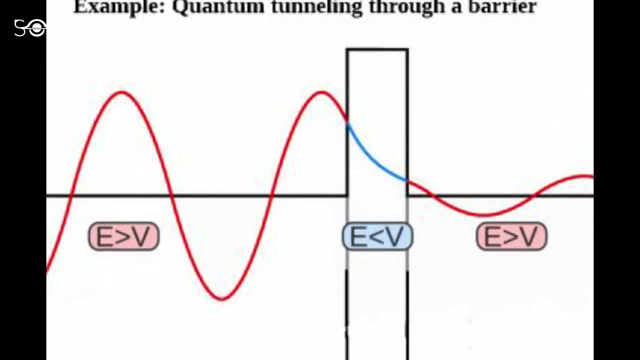 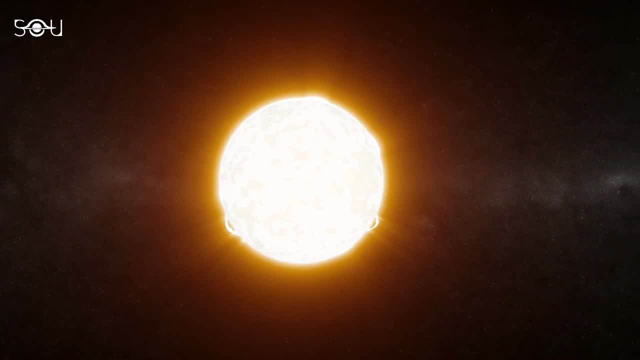 Technically speaking, a subatomic particle can pass through the potential barrier greater than its energy. Fun fact, this is the reason behind our existence. It is the basic principle involved in the production of nuclear energy in the core of the Sun. Number two, the wave-particle duality. in our daily lives or in the realm of classical physics, a?